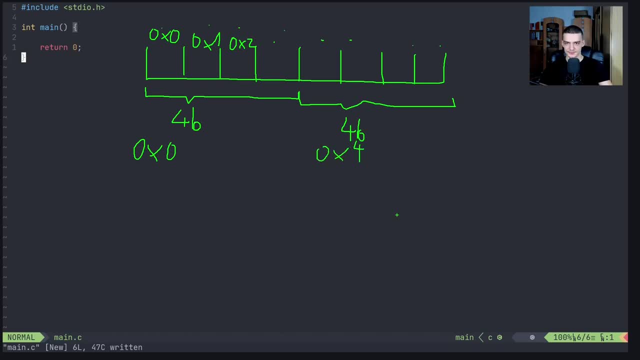 memory address zero x four in this case. So this is how basically memory addresses work. Now, in order to get these values in in C, what we need to do is we need to create such a variable, So, for example, int a equals 10.. And then we can use the addressing operator or the pointer operator. 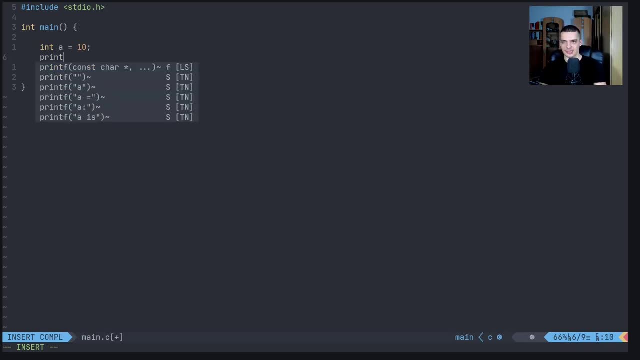 the referencing operator to print the actual memory address. So I can say: print f and now percent p for pointer backslash n and then we can pass and a. Now remember this n symbol here. this operator here was used already when we, when we. 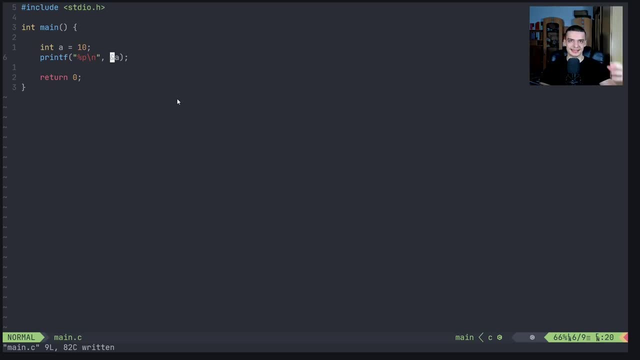 wanted to scan something. So when we wanted to take the user input and scan it into a variable, we use that to indicate that we're actually targeting not the variable itself but the memory address of this variable. So in this case we can run this: 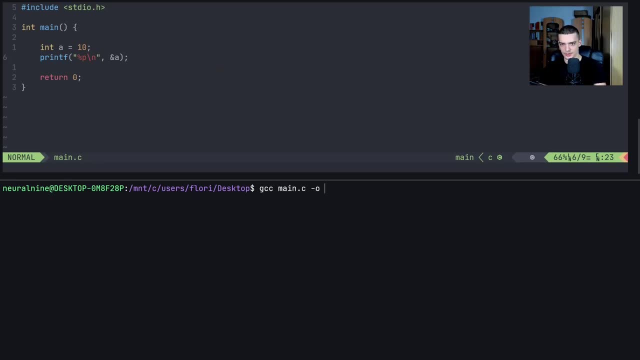 We can compile this GCC main, dot, C, O main, And when I now run this, we're going to see a memory address. So this is just one address. But what we're, what you're going to notice here, is that when I create a second integer with the value 20,, for example- and I copy this line and I also 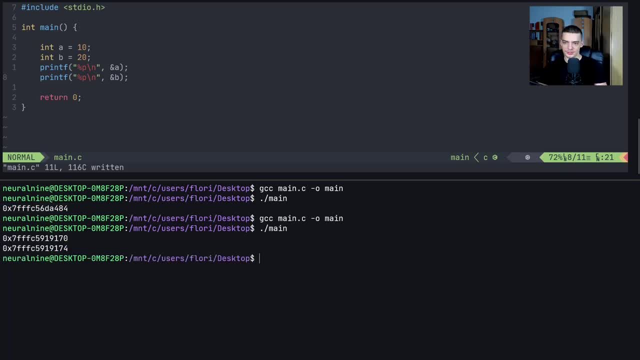 print the memory address of B. you're going to see that it's almost the same, but it's four bytes after this one. So you can see basically what we did with zero, x 00,, x one and so on. Here we have it in a different memory space, So this is. 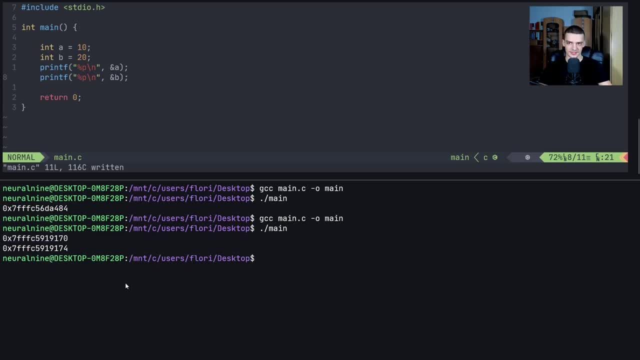 where we are at, And this is the first one. four bytes later we have this one, and so on and so forth. If I now choose to create a character instead of an integer, so char C equals a, for example, And then I print the address of C, Now in this case we won't actually see what I'm. 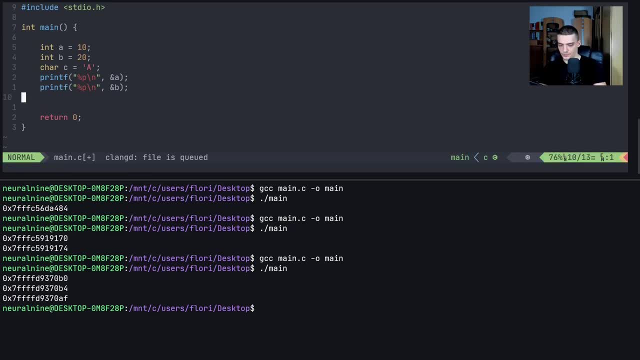 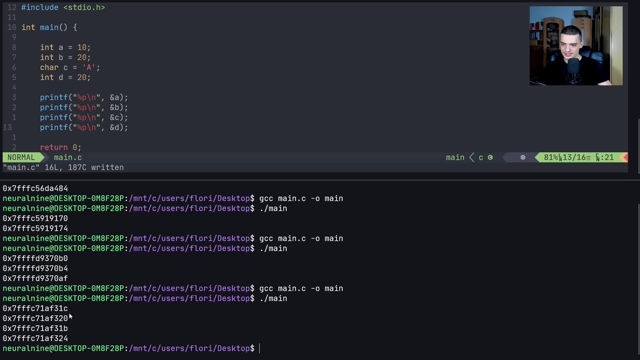 talking about. But if I, if I create another integer here- so int D equals 20,, for example- again, then I print this as well, you're going to see that there's a difference between integers and characters. So when I run this you can see from C to two zero. this is a jump of four. 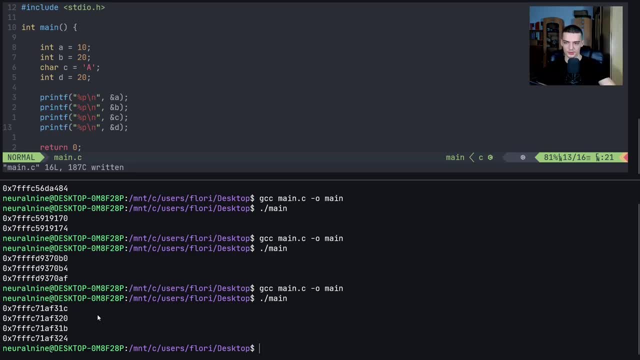 because we have C, then we have D, E, F and then we have zero. So this is a difference of four. We see that C is doing something else in the background here, So we can see that actually, in order to fit this more more beautifully into the memory, C has repositioned the allocation. 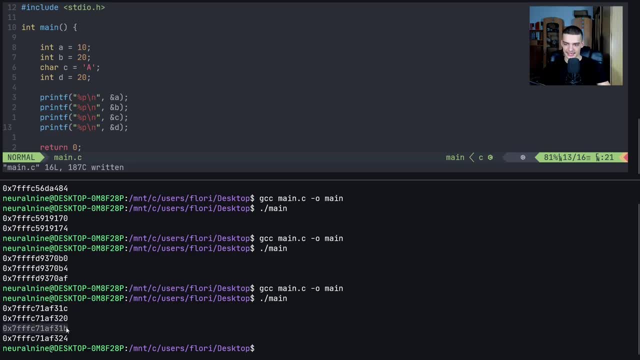 So you can see actually that the character is allocated first, but nevertheless you can see that after the character, one byte after that, the integer starts. so we don't have the order as I expected it here, Because we don't have first the integer, then the next integer, then the character. 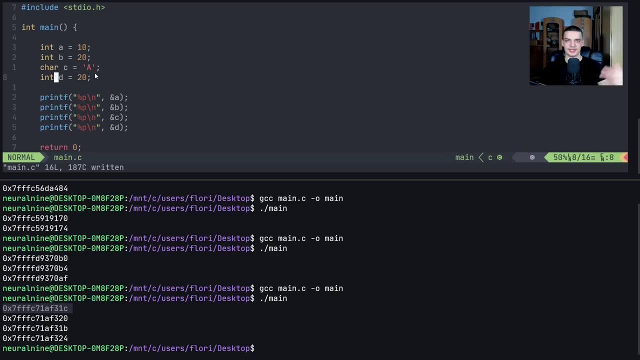 and then another integer. we have, We have the integer, We have the integer, we have the integer, the character first and then three integers. But the point that I wanted to make is still here, because we have this character here at this address and then one byte later. so from B to C, 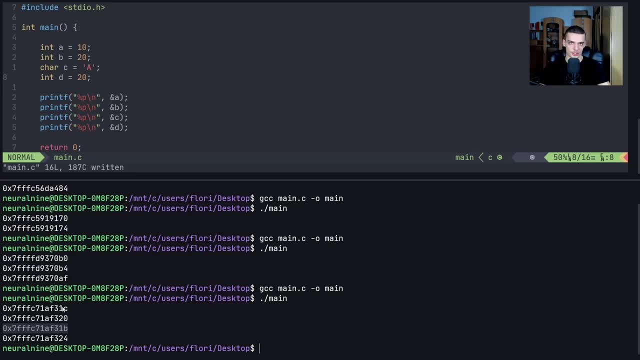 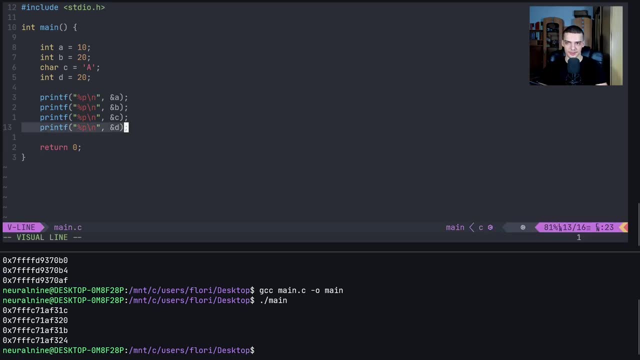 it's just one byte. we have the integer. this is because a character occupies one byte. So this is how you can look at the memory addresses. But those are not pointers yet. those are just memory addresses. A pointer is a variable or an object that points to the memory address of something. So 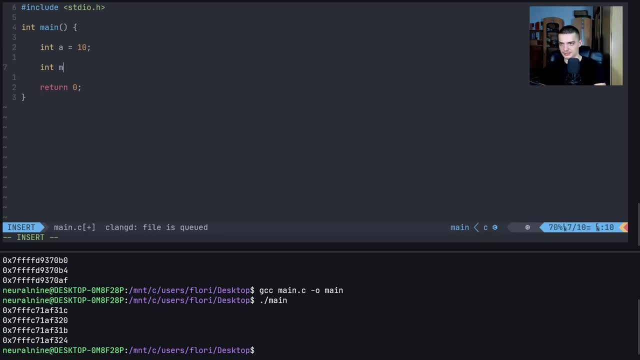 for example, we can have an integer pointer, we can call this int my pointer, And then we add this star symbol here, this pointer, pointer symbol or pointer operator. you could say: and usually I like to do it here, Or actually I think we need to do it there, So we have an integer pointer to 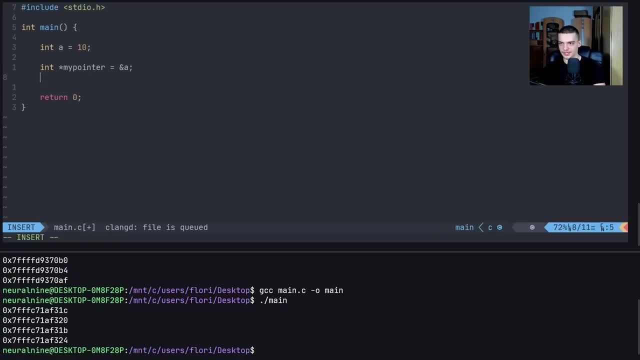 the memory address of a. this is now a variable, So we can go ahead now and say: print f, percent, p backslash n of my pointer And we're going to get the same result here. There you go, So you can see, of course, different. 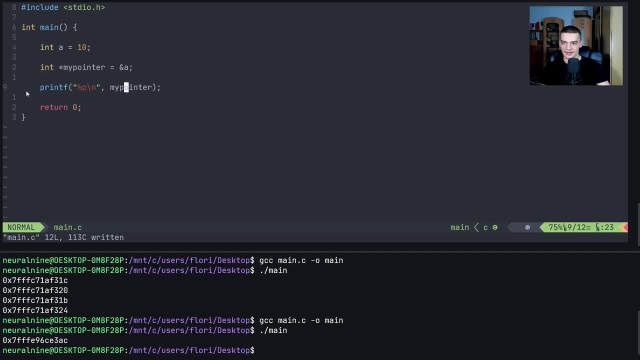 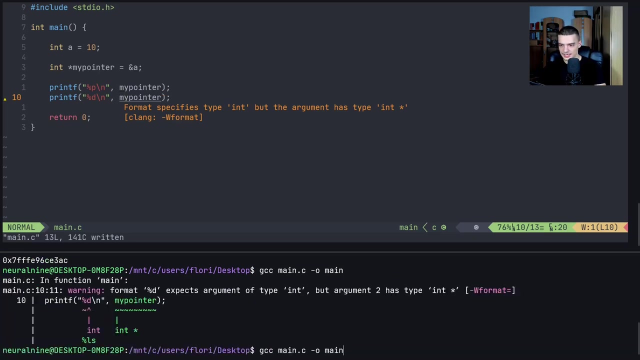 memory address and all that, But this is now an entity or a thing that points to the memory address of a. Now I can also try and print this as a number, But you can see here that I get the warning that I'm trying to print an integer even though I'm passing a pointer. not even sure if 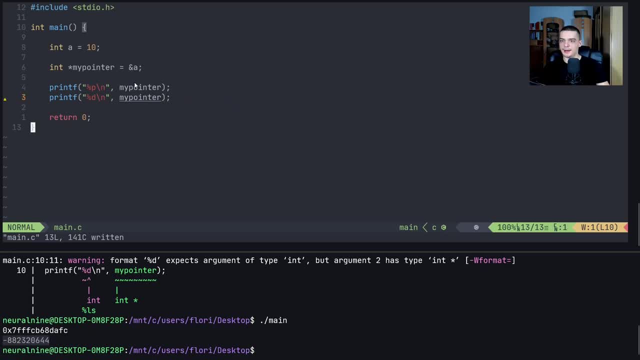 this is going to run properly. okay, we get something here. But what we can do is we can do, since we already had the pointer in the memory address. obviously, and it's a pointer as well, we can de reference a pointer, And what we can do here after that is faith that I want to present. 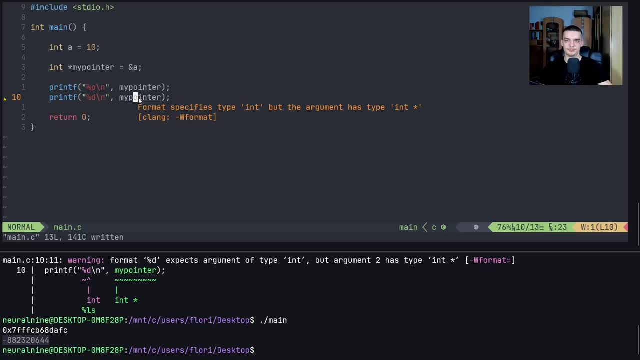 alias, so we can praise it. We can say file address as aů, just a for the name of our container, And then we've got all our entries, all the sheet numbers, all ready in a row. we can do this in a way that gives us a very clear image to be able to understand. 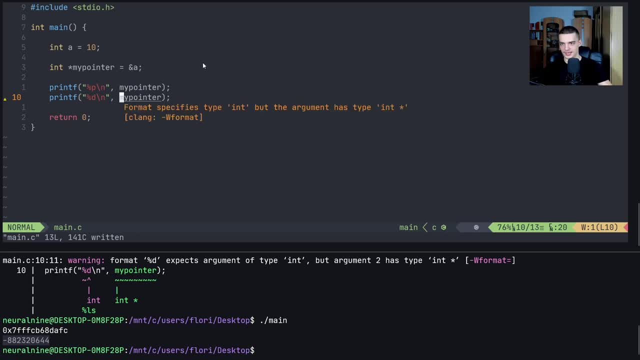 if the pointer is or not a value, To make it clear that says earth uniform is milk, emotion or the word person. And I can also do, And again when I was looking for this, HARVEST, то же. let me justреfer〜 the pointer: let's try a bit more here in the value set, let's try to get. 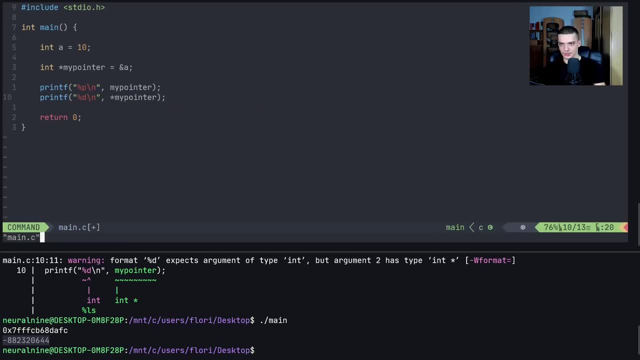 the value that is stored at the memory address of a that it is pointing to, because this operator here the star symbol to dereference the pointer And in this case this gives me an integer And you can see that I get 10 as a result. So this is how pointers essentially work. 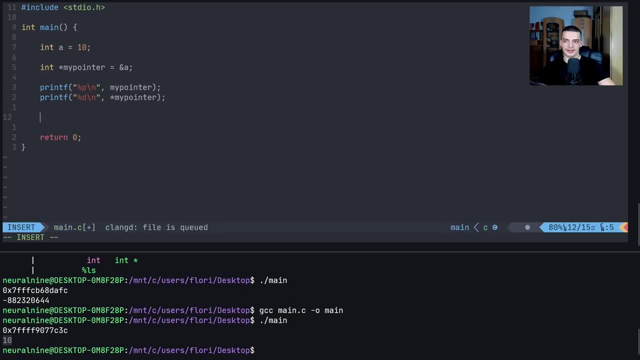 We can also use that dereferencing here to to change the value of a, so I can go ahead and say my pointer first of all. if I just do my pointer something, it has to be another address, So I have to pass here another memory address. but I can also dereference here So I can say my pointer. 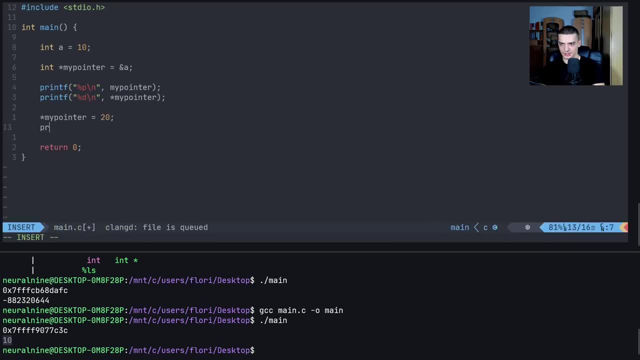 dereferenced equals 20.. And then I can just go ahead and say: print f, percent d, backslash n: a. So I'm not even printing the pointer, I'm printing a And you can see that this changes the value of a. So this operation here, this means that we're changing the content at the memory address. 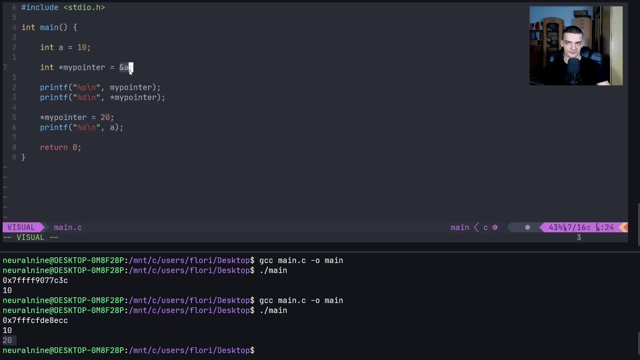 whatever, And this memory address, whatever is the memory address of a, and we change it to 20, then we print a and we can see that a in fact has to value 20.. Here we cannot do that with an ordinary variable. So I cannot just say in copy equals a, and then copy equals I know 300, and then print f. 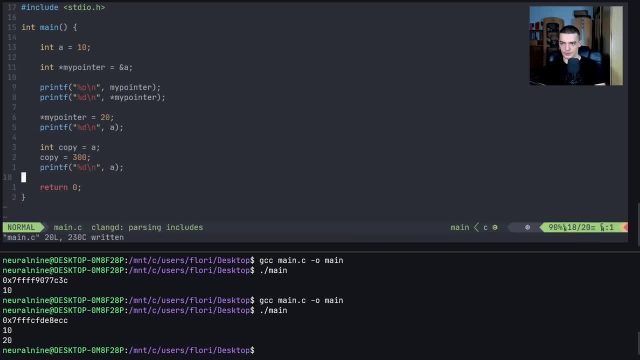 a, this is not going to work. So making a copy is not the same thing as using a pointer, dereferencing it and changing the content of the memory, of the memory address. So this is a difference. This is something that you cannot do just with basic copies. Now, one thing I want to: 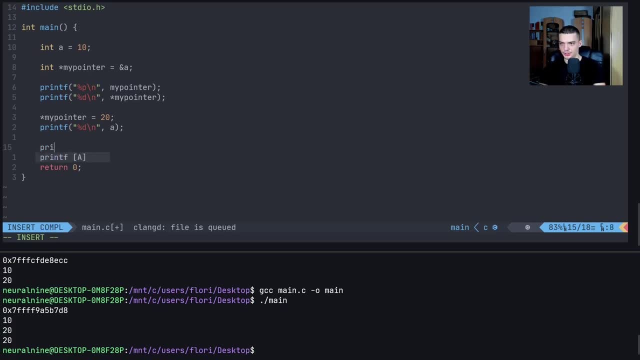 show you. here is the size of a pointer, because the size of a pointer can be printed here again with percent ld backslash n. then size of my pointer, the actual pointer, And you can see that in this case here it has eight bytes. So the size of a. 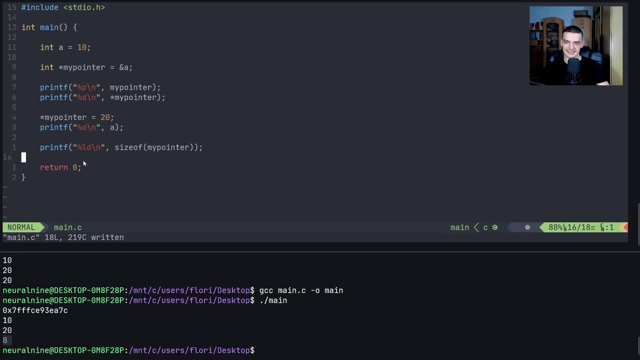 pointer has eight bytes. Why does it have eight bytes? it doesn't have eight bytes because the pointer is so complicated. It has eight bytes because we're operating on a 64 bit system. On a 64 bit system, the memory addresses have 64 bit, aka eight bytes. So 64 divided by eight is 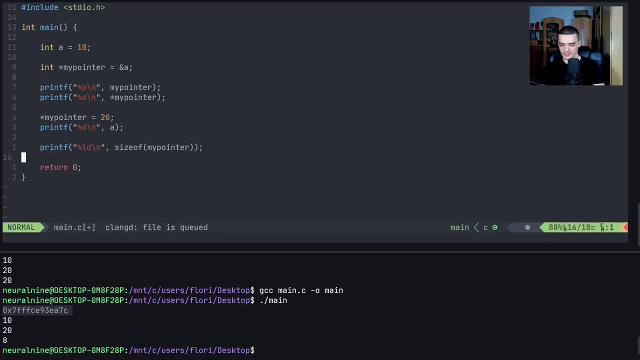 eight. So we have eight bytes. on a 32 bit system we should have four bytes for a pointer. So the size of a pointer is going to be eight bytes, just because the memory address space is 64 bit. So this is important. What else can we do here? we can also, of course. this is important. 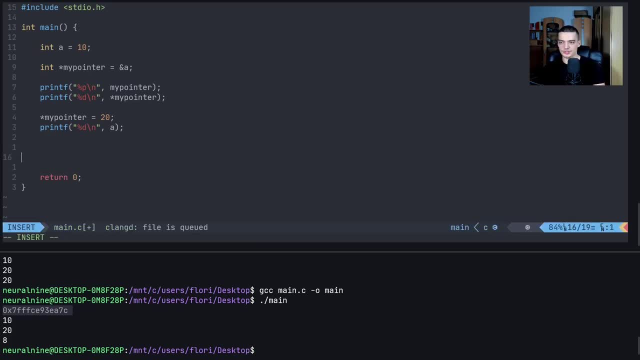 I didn't mention this here. the pointer itself, of course, is all also stored in the memory. the pointer is not just some magical thing floating around in the in the code. it's actually another thing stored in the memory. So actually we can print a couple of. 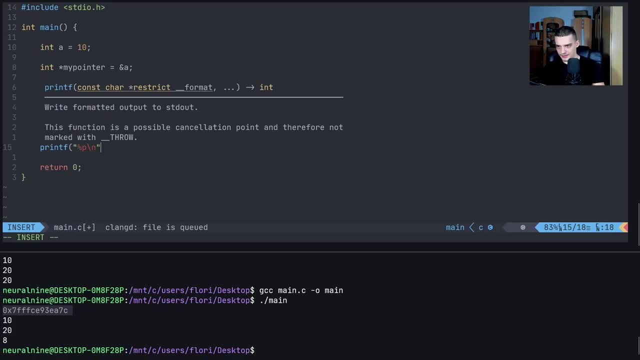 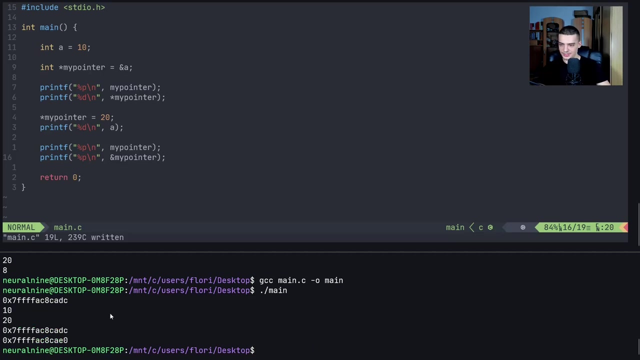 things here. we can print the address that the pointer is pointing to, So we can do that which I actually did above, but I can also print the memory address of the pointer itself, So you can see that the pointer itself is stored in the memory And of course this means that we 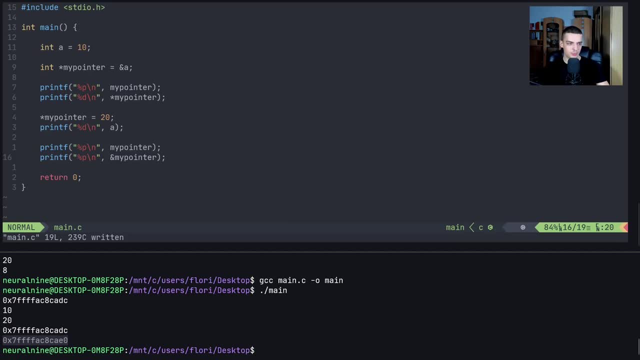 can create pointer pointers. we can create pointers that point to pointers. So we can go ahead and say Int and then star, star, p, ptr, So pointer pointer basically equals and my pointer, and this then creates a pointer that points to the memory address of the pointer. Now, don't be. 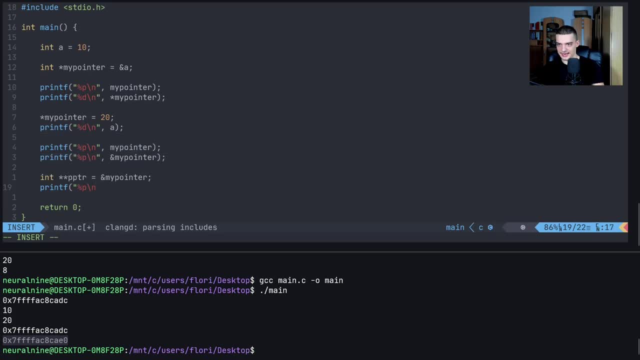 confused here. This is all very abstract. you cannot see right now why this is relevant or important, But this is how we work in C. we have to do this manually because it depends. It is oftentimes important what we actually pass. are we passing a pointer? Are we passing a variable copy? we need to know about. 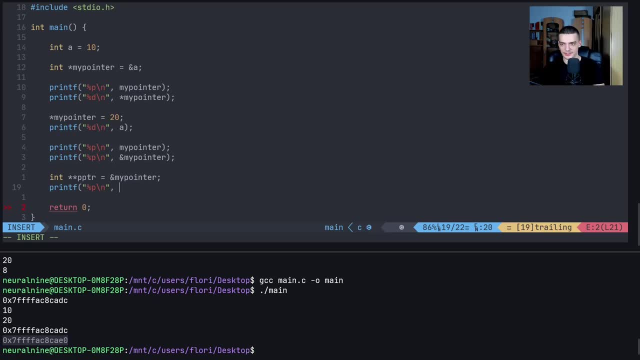 that stuff And Python. we do not know about that stuff because it's not really relevant to us. In Java Also, we don't know about that stuff. Java works with pointers, but we don't see the pointers in C. we need to actually care about this. So here I can pass again pptr, which is 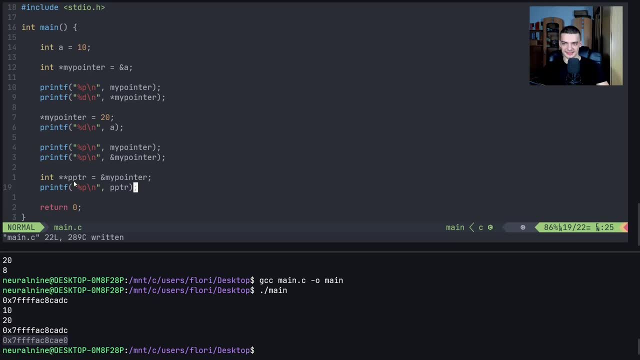 a pointer to the pointer. And guess what? we're not going to do this endlessly here, But this thing here is again stored in a memory, So we can point to it as well. We can do this over and over again. we can point, we can point to pointers, of pointers, of pointers and so on, But we can also: 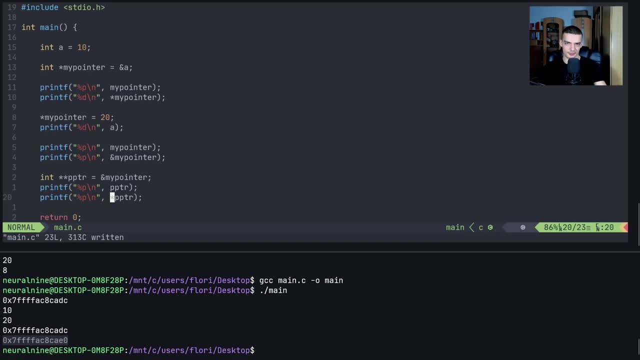 dereference the pointer, and it's still going to be a pointer because it is the pointer, my pointer, And then, last but not least, we can also get the value by dereferencing it twice, So we can dereference the pointer and then dereference the pointer that the pointer 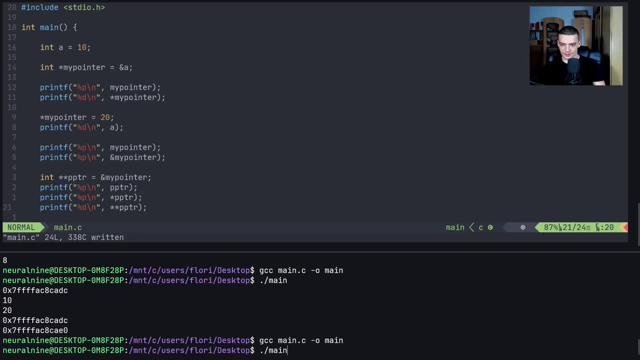 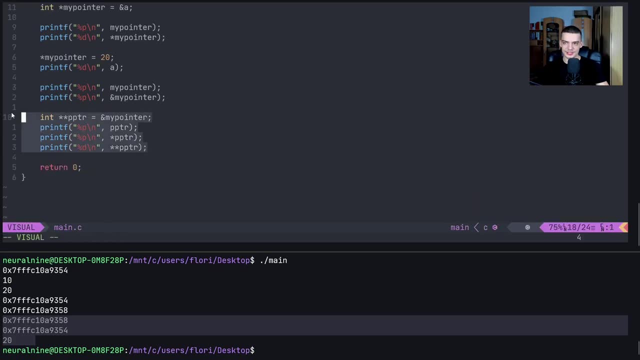 pointed to getting more and more complicated here, isn't it? So there you go, you can see what I'm talking about here. Again, this is just some theoretical background. you don't need to understand everything exactly and why you need it. Essentially, we have things in C that allow. 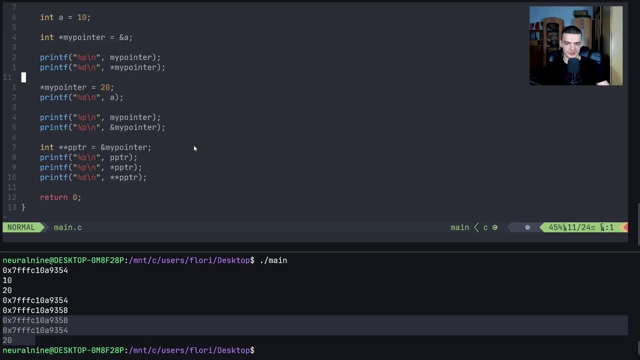 us to store the memory addresses of objects And we can use those to actually pass the precise pointers, the precise addresses, which is important because sometimes we have functions like the scanf function and we can only pass the pointers. So we can only pass the pointers. 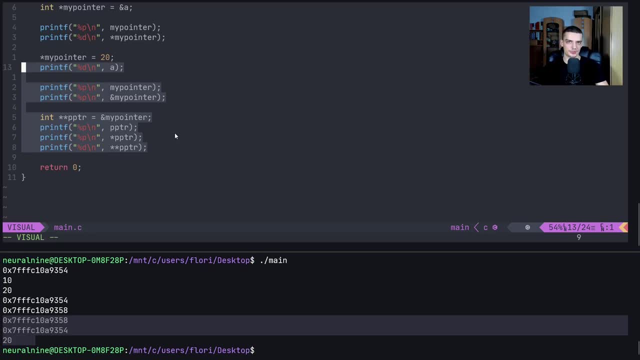 And not just variables, because variables have values and pointers have memory addresses that we can change. And one thing that is also interesting to notice here is that arrays essentially can be treated as some sort of pointer. So an array is essentially just a pointer to the first position. 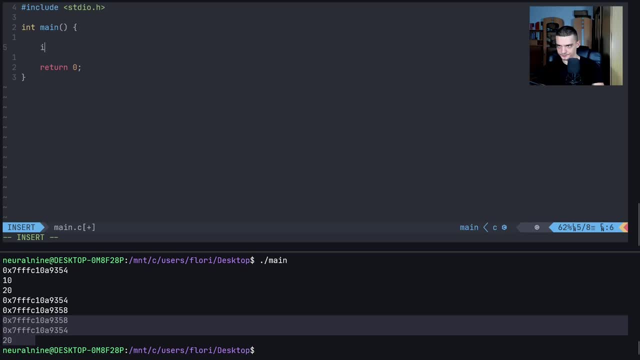 So if we have, for example, an array, an integer array, with, let's say, 100, there you go, with 100 values. here this array is essentially just a pointer. So I can go ahead and say: print f, percent, p, backslash n, and I just have to pass the array. I don't even have to pass. 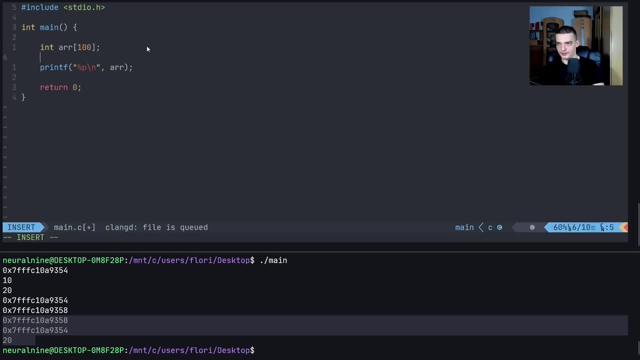 the n symbol here with every other variable. If I have for example here I don't know- a floating point, number f, And I want to print a pointer here, I cannot just pass f right, this doesn't work because that is not a pointer, But array itself is a pointer. So this: 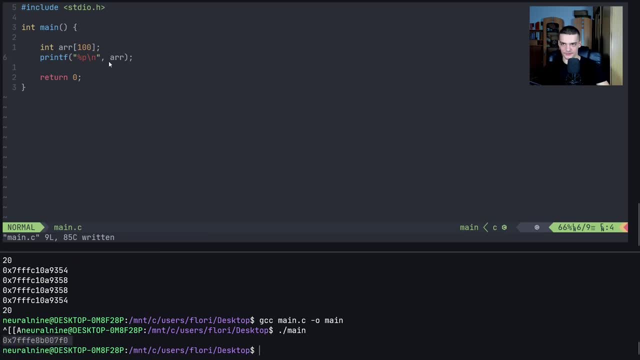 works here You can see that this is the address of the starting of the starting elements. So essentially we can use that to to get the beginning memory address. So an array itself is just the address of the beginning of the whole thing, because an array we have here, an array with a couple of 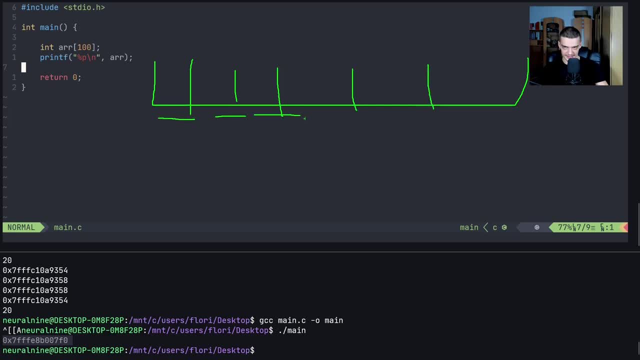 slots here. let's say, all these are four bytes because it is an integer array. This here is index zero, And if we get the pointer of an array we get the address of the first position. basically, we can also go ahead and actually just 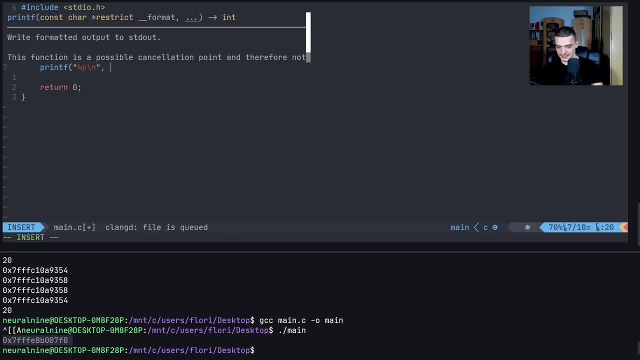 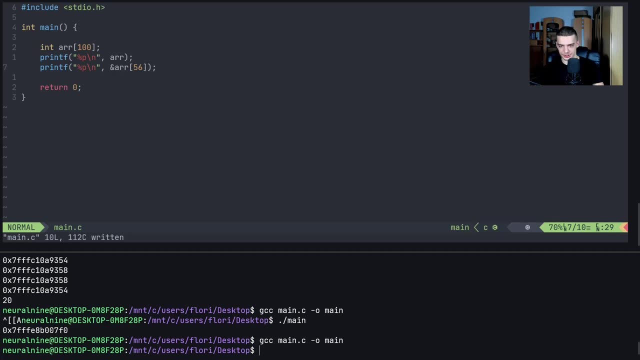 print the pointer of a certain position. So we can go ahead and say and array 56,, for example, and then we're going to get the memory address of that particular position. And here I'm not going to do the calculation right now, But this should be 56 times four bytes after this address. 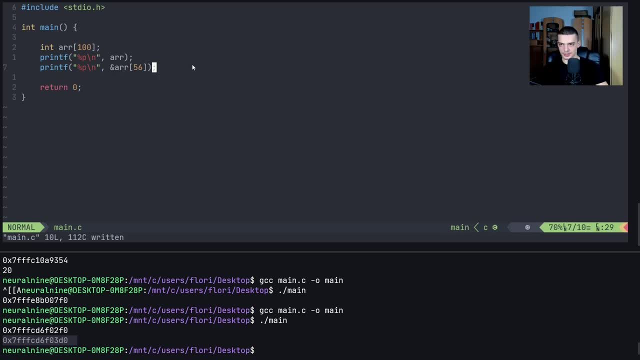 here. So that should be the difference. Just a nice thing to know on the side that arrays are actually just pointers. this can be important when programming. Besides that, we should also talk about pointer arithmetics. pointer arithmetics are actually quite interesting, Because once we have a pointer, 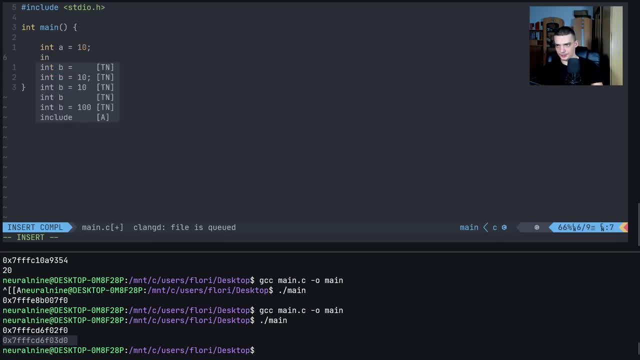 again, let's create a variable: A equals 10,. we can create a pointer here in PTR is going to point to a. we can also go ahead and do pointer arithmetics: a pointer can be increased, a pointer can be multiplied and so on. So essentially I can go ahead. 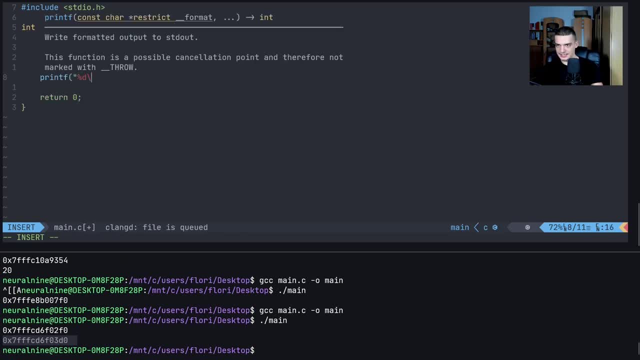 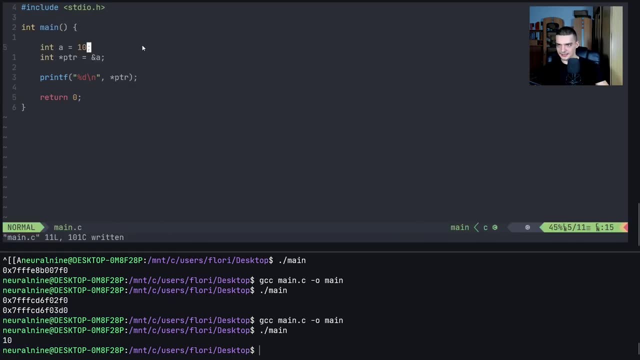 here and say: print f, percent d backslash n, and I can dereference the pointer here to get the actual value of a. And then I can also go ahead and create another variable: b equals 20.. And I can say ptr plus, plus without dereferencing. So I'm not actually increasing the a by one, I'm increasing 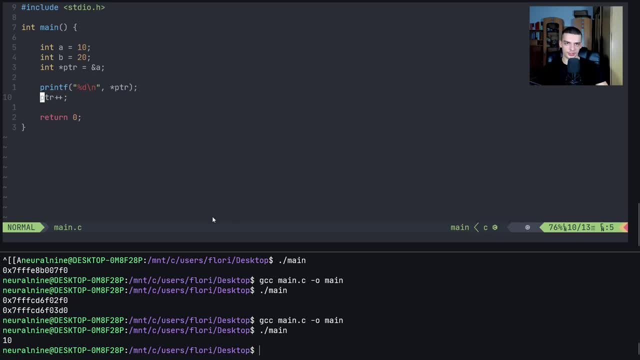 the value of the pointer by one. increasing the value of the pointer means jumping one space, or one one memory address space, to the right, if you want, So to the next, to the next area, which means, in terms of an integer, adding four bytes. if you're not dealing with integers, if you're dealing 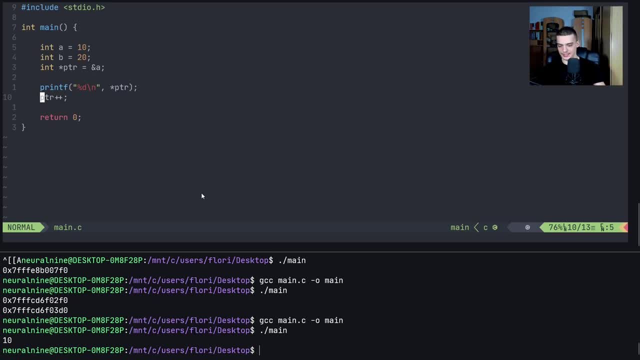 with characters. this is one byte at least- with this compiler in this system. So if I actually go ahead and copy this, I think at least that I should get. Yeah, there you go. B is a result here. So I just changed the pointer here by increasing it And then I dereferenced it and 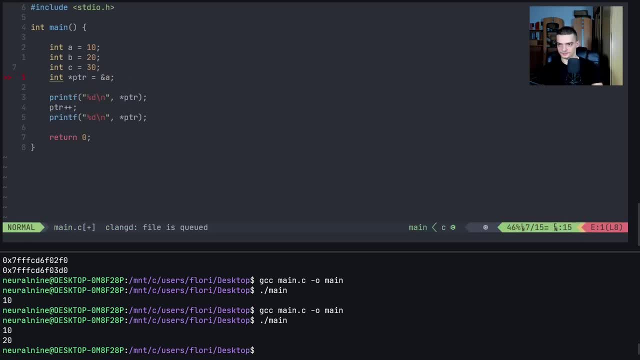 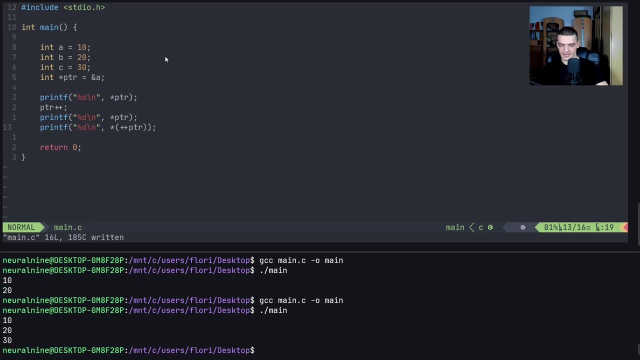 got the result. Now, if I add C here, I can also print it directly. So I can say: okay, get the pointer plus plus the pointer. So increase the pointer by one, then dereference it, And this should give us 30 here, as you can see. So that's essentially the basic idea. 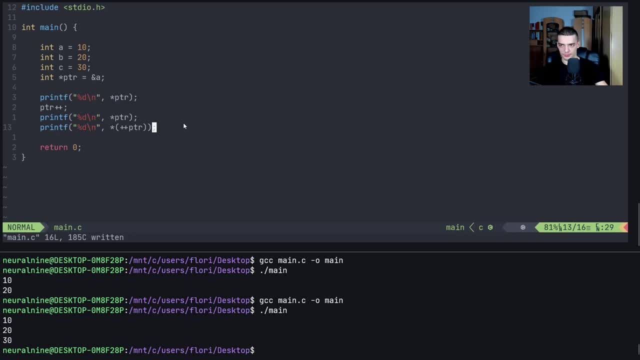 behind, behind increasing pointers, we jump one address. I can also do this right away, So we can actually do plus equals two here. this is not going to increase the pointer by two, it's going to increase the pointer by eight. So it's not going to jump two bytes, it's going to jump a. 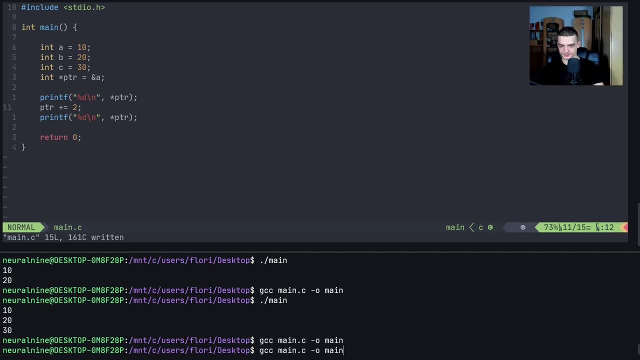 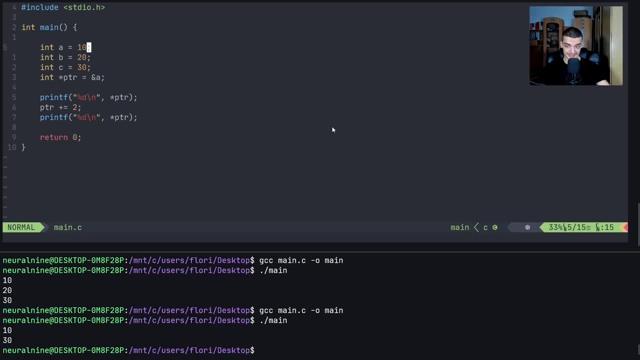 byte. So two, two times an integer size. There you go. So we skip the 20. And we jump immediately to the 30. Since it's in the neighboring, neighboring memory space. And of course we can use all that to also jump back, So I can say pointer minus, minus. I can then print it again. 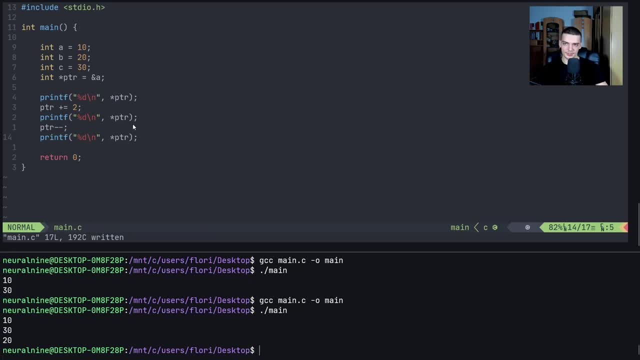 and then we should see 20 afterwards. So a very simple thing. This is how we can jump with pointers, how we can increase them, decrease them, and so on. We can, of course, also go out of the memory space. So I can say: plus equals eight, And if my program does not crash, we're going to get 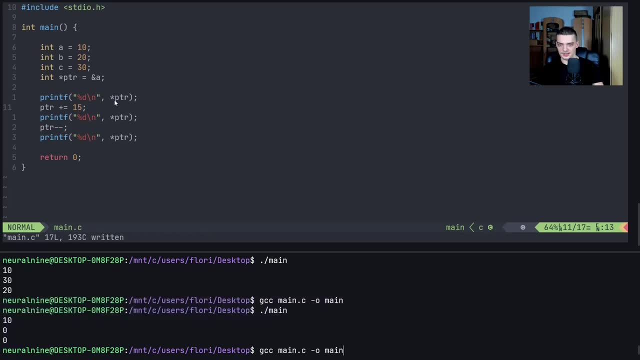 some random values here. I can also change this to 15.. Maybe, I don't know, maybe it's going to be counter some interesting values here. The problem is when you choose to write because you know. now I jumped with a pointer to some memory address. I don't know what's there, And if I then go ahead, 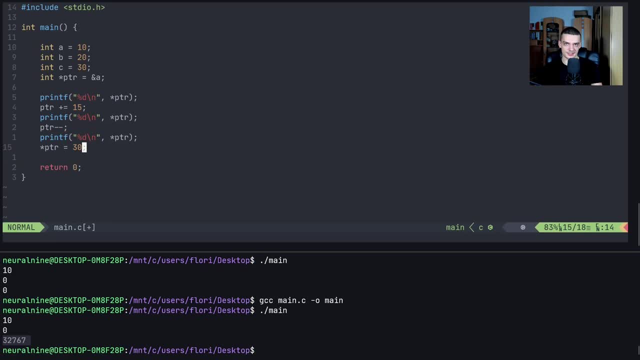 dereference it and assign something to it. we don't know what happens. Best case, the whole application crashes And that's it. Worst case, I do something that I don't even realize I did, especially if this is a serious tool. I have created some severe security issue here, So 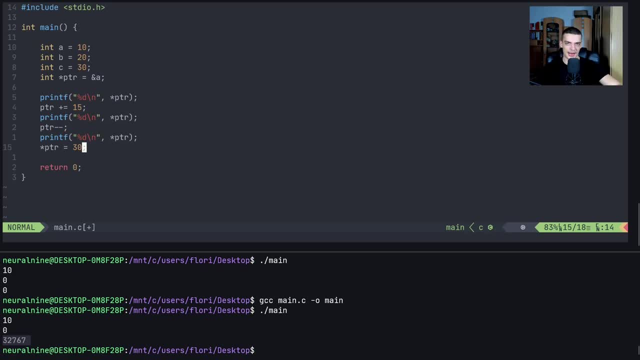 this is something that you should definitely avoid. Remember: you can go out of the, out of the targeted memory space. you can do whatever you want. you can override, jump back addresses, which makes it, of course, very vulnerable to buffer flow, buffer overflow attacks. So you don't want to do that, But this is essentially how we do. pointer: 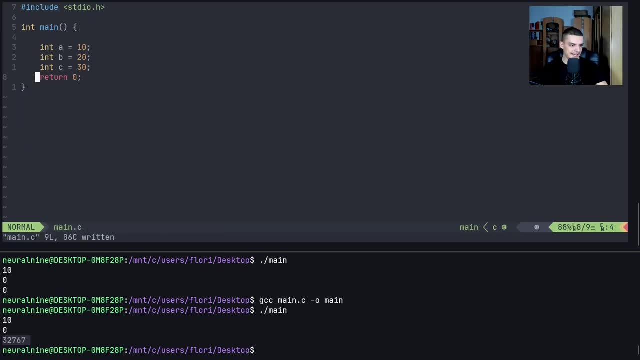 arithmetics, That's that. So then we also have: how can we basically iterate via arrays? So this goes back to the point that arrays are essentially just pointers to the first position. we can have, for example, int numbers, 100.. And then I can just say: okay, the first, the first number. 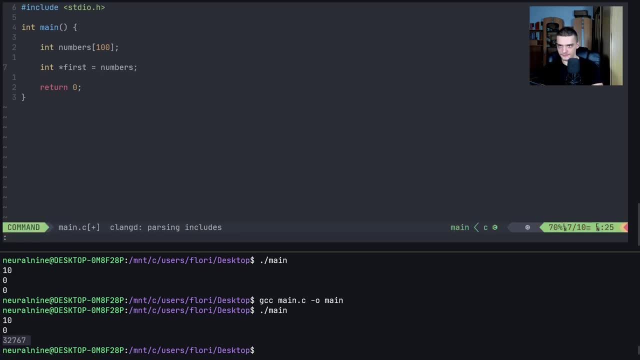 the pointer to the first position is essentially just numbers itself, And then we can do a full loop. we can say: for int I equals zero, I is less than 100, I plus plus. There you go, And here we can then set the value. So we can say: take the position of the. 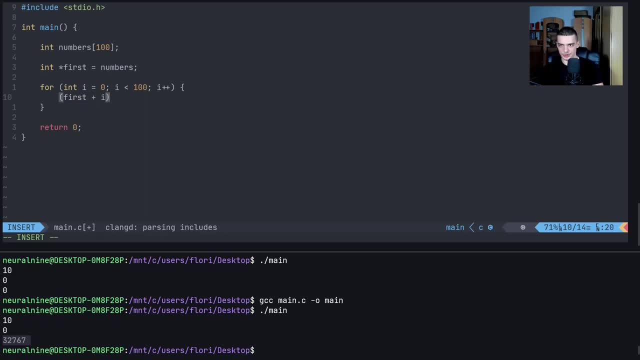 first of the first number, add I to it. So jump I positions, dereference that thing and add something to it. For example, I times 20. I don't know. So again, we take the first position. the first position always stays the same. we add I to it, which means that we jump in the first. 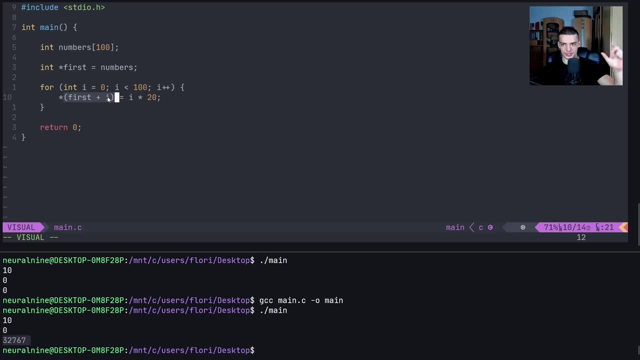 iteration, nothing. we stay at the first position And the next we jump four bytes, then we jump eight bytes, 12 bytes, and so on, And we always set another value, And then we can also go ahead and print these values with another loop. So for: in I equals zero, I being less than 100, I plus. 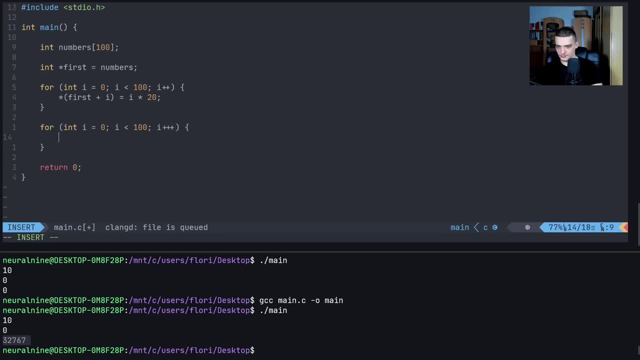 plus, we can just print. print f, percent, d, backslash, n of numbers. What's the problem here? Oh there, you go, Compile, run And you can see the values here. So this is how you can do that. Then a couple of things we should talk about is something called. 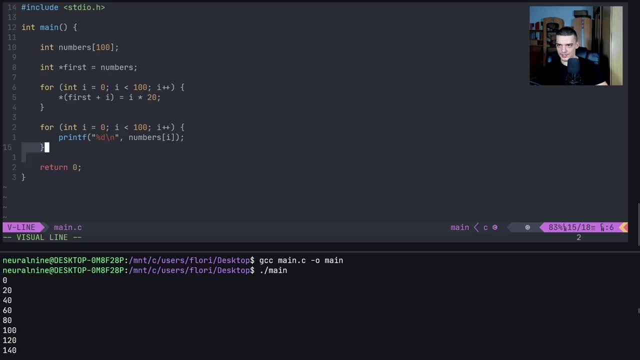 the null value. I'm not sure if we discussed a null value already. I think not. Null is essentially just in C, it's just a macro or a constant that represents zero. In other languages null stands for basically nothing is here, And in C it should also stand for that. But the practical 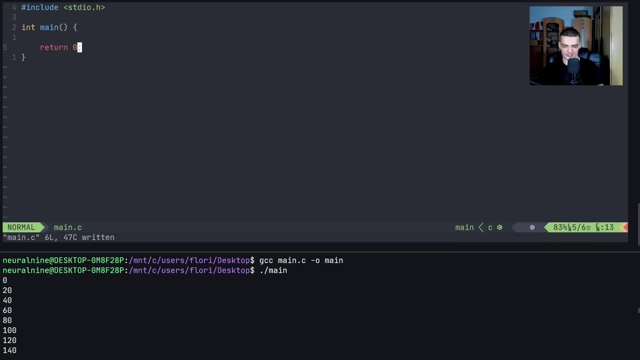 thing is, or the reality is, that null is essentially just zero. So if you say, for example, here integer pointer points to null, this, basically you do that to say, okay, this pointer points nowhere. However, null is essentially just another way of saying zero. So this is basically the same, I think. 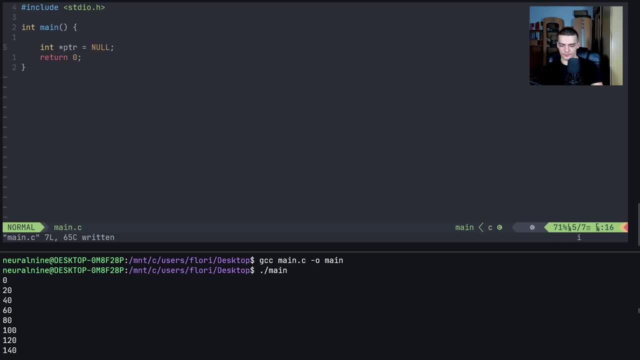 that the only difference is that it's how turned into a void pointer. I think it's typecasted to avoid avoid pointer, But essentially it's just a zero in C in. in C++ we have the null PTR, which works a little bit differently. 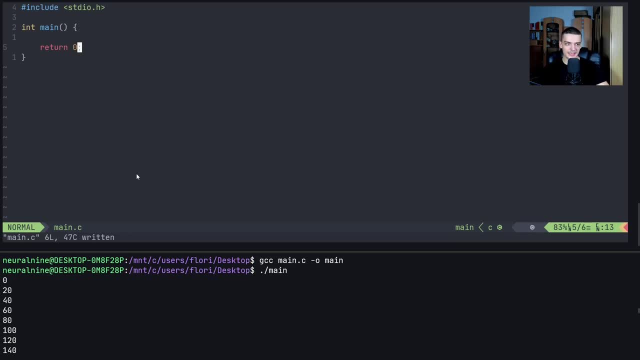 but we don't have objects and so on, and see Speaking of of void pointers. we can use void pointers to keep the data type of the thing that we point to flexible. So we can say: void pointer, VP. here is, for example, the pointer to a. we don't have a, a could be an. 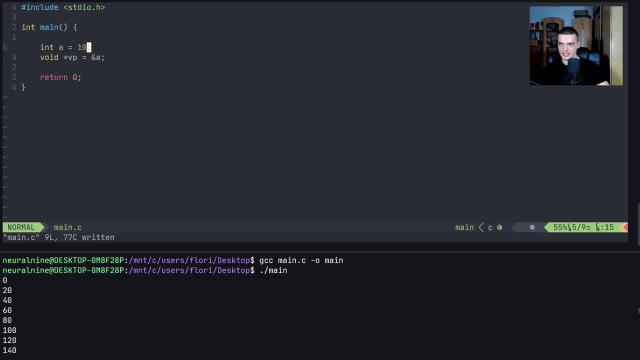 integer. So this definitely works. But we can also point to different things, right. So we can. we can point with a void pointer to essentially everything, And then we can also print this. So if I say print f d backslash n, and if I now want to dereference the pointer, we have to do that using 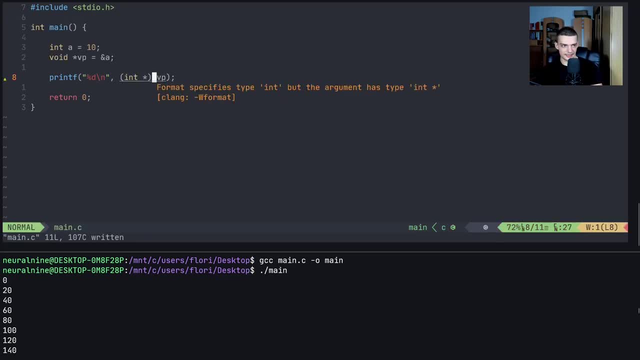 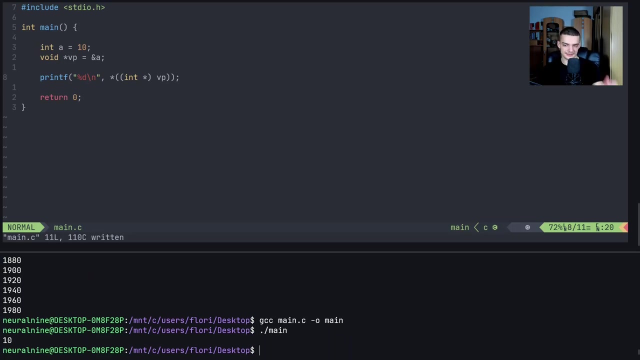 typecasting, So I would have to do it like that And then- or actually did I do it, Oh sorry. we need to typecast first into a, an integer pointer, and then we need to dereference it to work. But this is how you would do. that can be quite useful, but we don't need this for this. 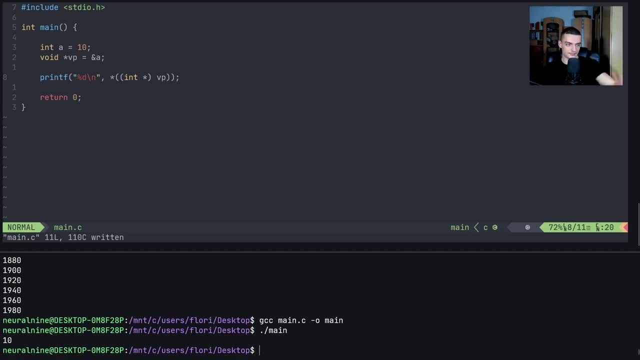 beginner level that we're at right now. So this is just something that you know. you should maybe know that it's possible. Another thing is that I think there's an interesting thing if we have something like a character pointer and this character. 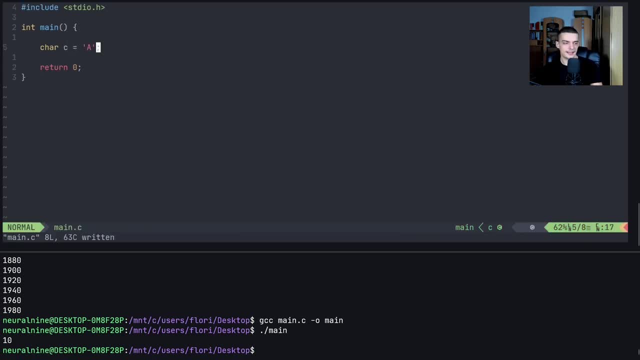 is for a character actually, and this character is a, and then we have: we want to print the pointer to see. I think was it like that? I think in C we actually don't have the issue that much, But in C++ we have the issue because we can also interpret this as a string. That's the problem. 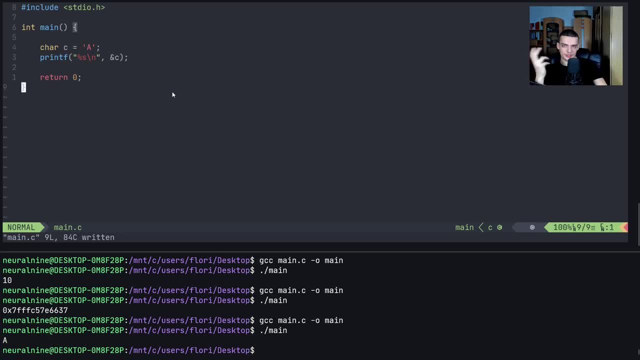 here, Because essentially, what a string is? we already talked about this. a string is a pointer to the first position. So if I say that the pointer to C has to be interpreted as a string, essentially this is going to treat and see as a, as a string, as a character array, and it's going to 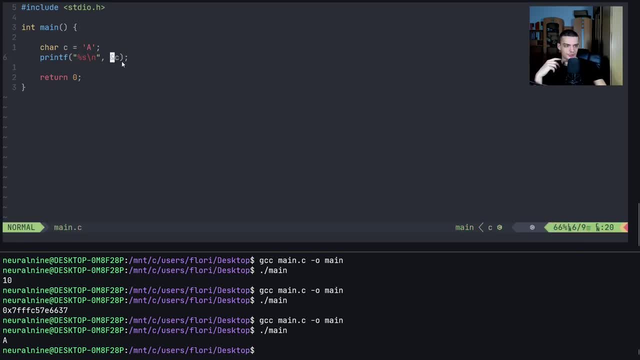 look for the null terminator and just print. So this is just also one thing to know. this episode is quite theoretical. we learn a lot, we don't really do a lot, But this is something that you always need to keep in mind when you work with things in C++. 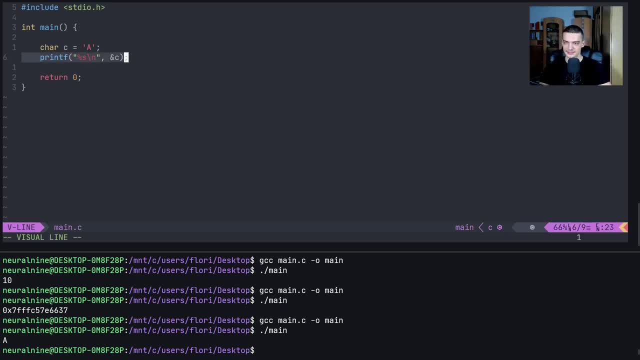 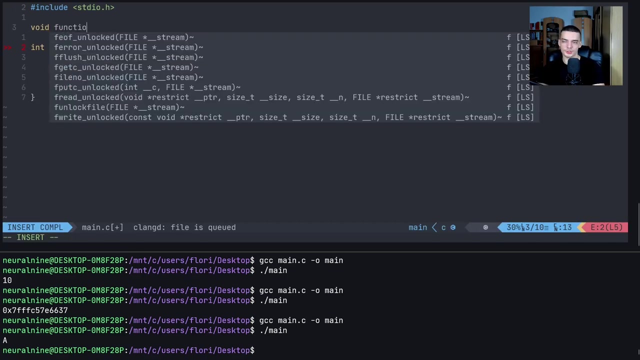 And the last thing I want to show you for today's video is how we can work with function pointers. So we have basically a pointer to a function. let's say we have, let's define a function here. Void my function. Actually, let me, let me do it like in my example here. Let me call them function one. 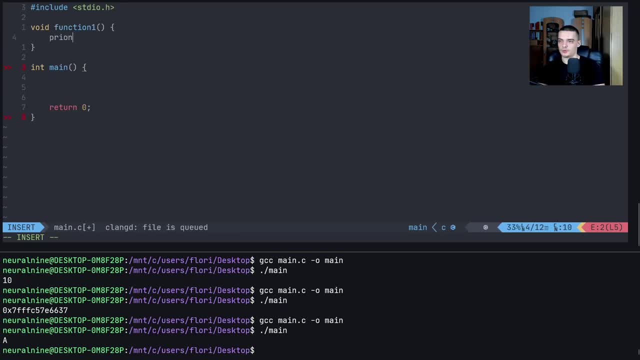 And we're going to print with function one, function one, backslash n, And we're going to copy this. we're going to paste this function two, function two, And now we can use a void pointer to keep it flexible. which one we're actually? 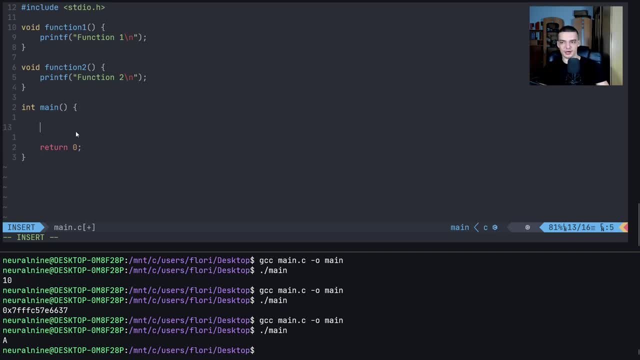 selecting, And then we can just execute the void pointer, And depending on the variable, we can just do that, So we can say void, And then in parentheses we can use this operator here again and call this my function, for example. 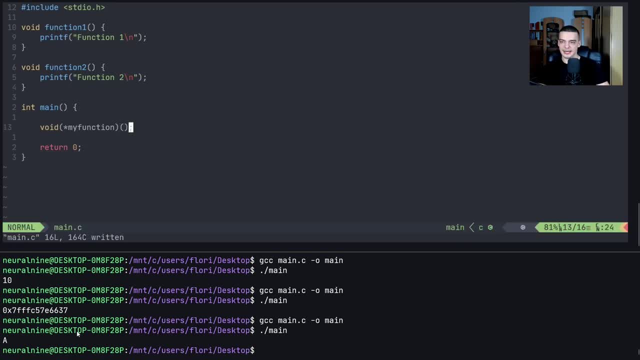 Like that And this essentially creates this, this void pointer, void function pointer. The important thing is that it has to have the exact same signature. we cannot have multiple parameters here and not have them here. we cannot have a different return value. it has to be the same.